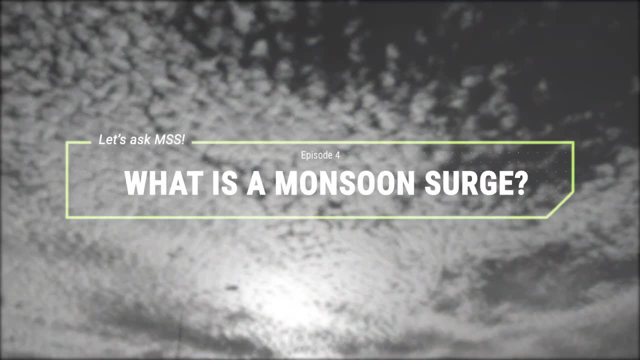 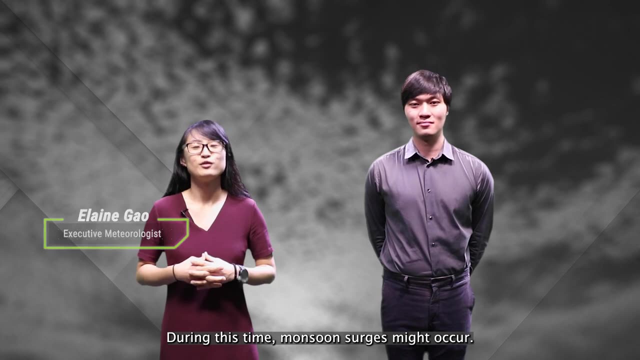 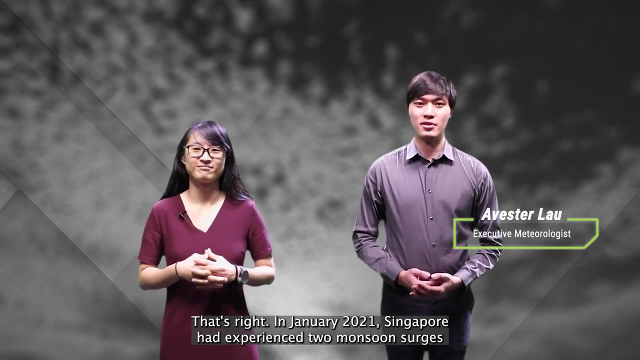 The Sembil usually marks the start of Singapore's northeast monsoon season. During this time, monsoon surges might occur. That's right. In January 2021,, Singapore had experienced two monsoon surges, which resulted in continuous rain, strong winds and cooler weather. 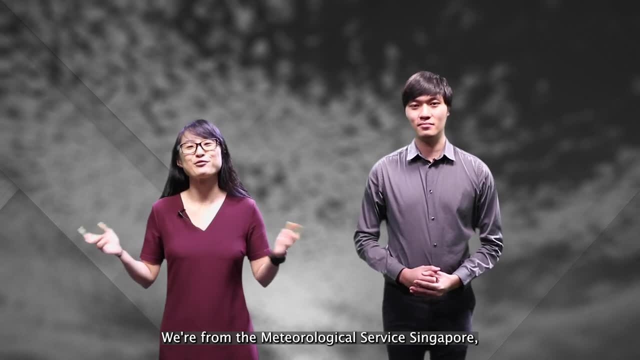 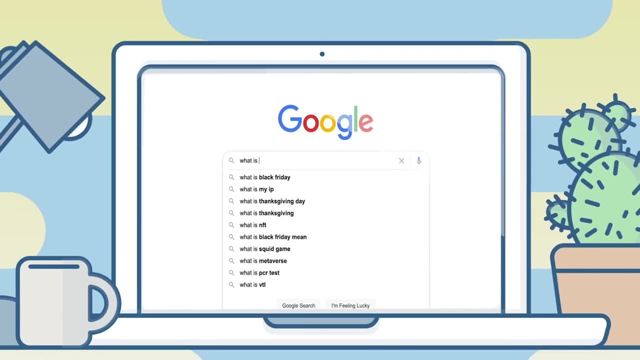 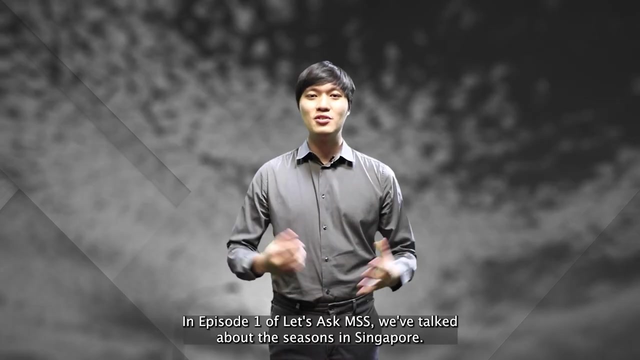 Hello, I'm Elaine And I'm Avestor. We're from the Meteorological Service, Singapore and in this episode of Let's Ask MSS, we investigate what is a monsoon surge. In episode one of Let's Ask MSS, we've talked about the seasons in Singapore. 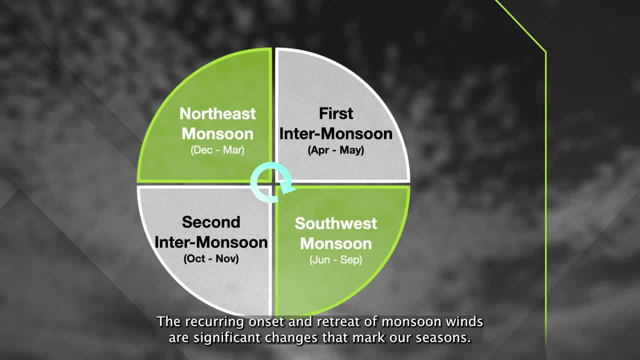 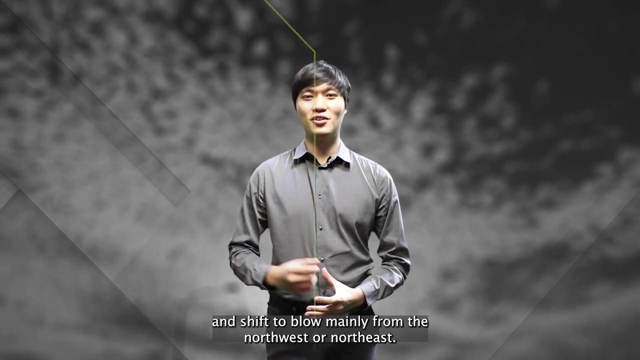 The recurring onset and retreat of monsoon winds are significant changes that mark our seasons. Typically, between December and early March, Singapore experiences the northeast monsoon. During this time, the prevailing winds strengthen and shift to blow mainly from the northwest or northeast. 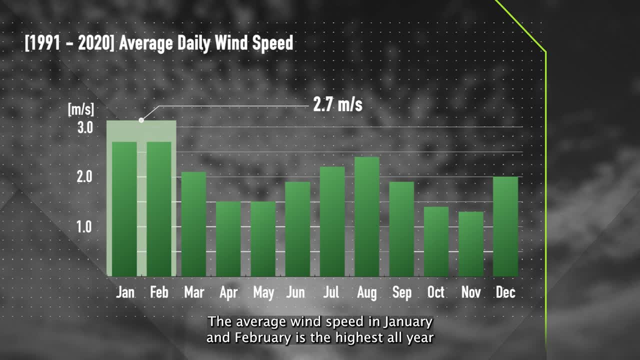 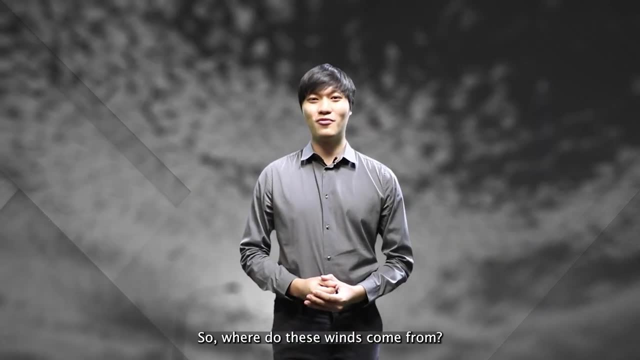 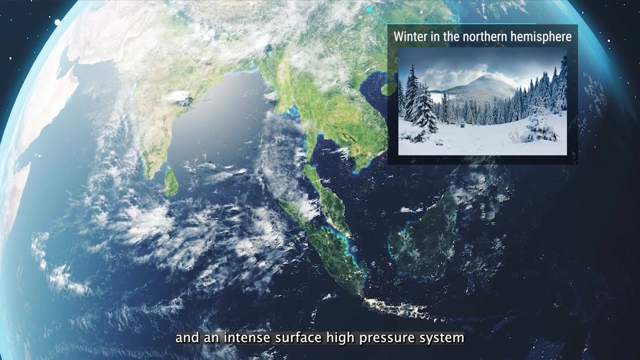 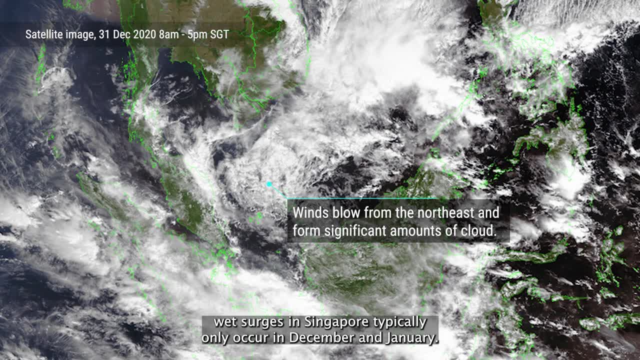 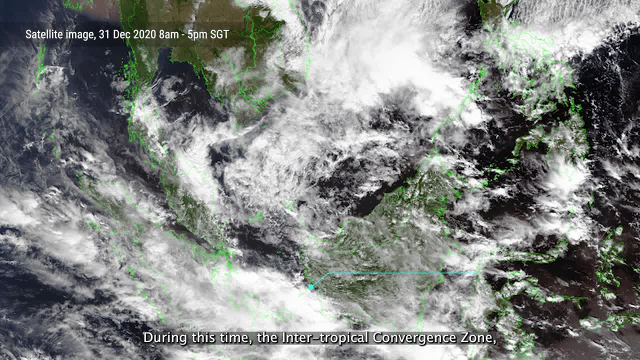 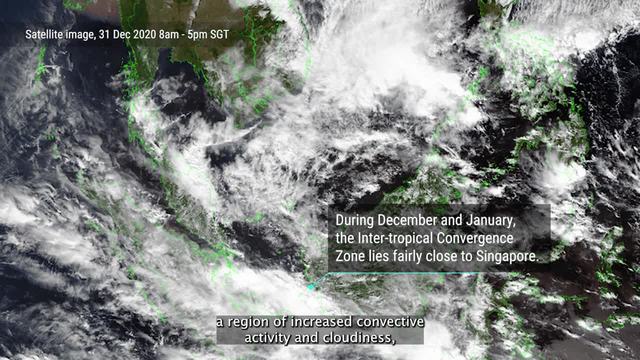 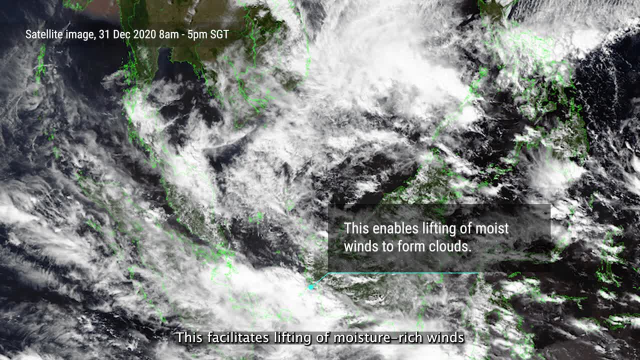 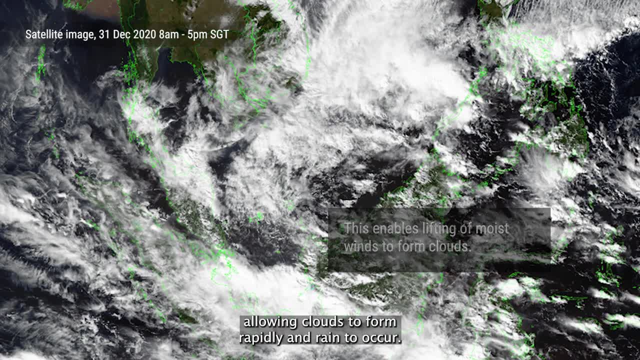 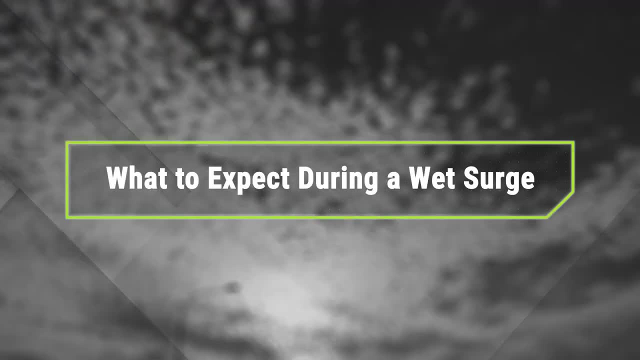 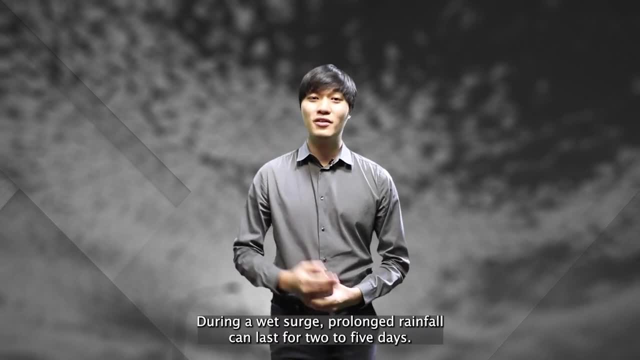 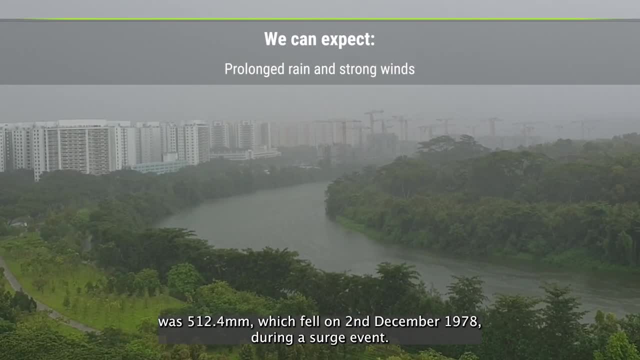 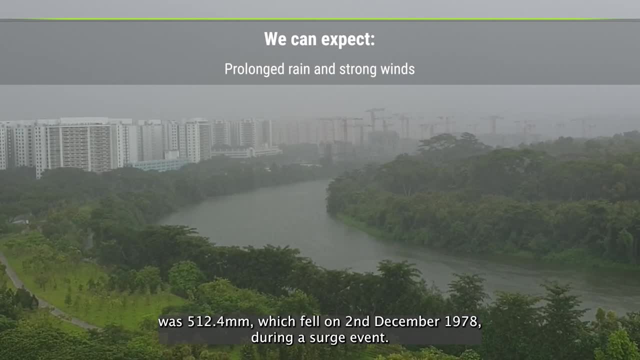 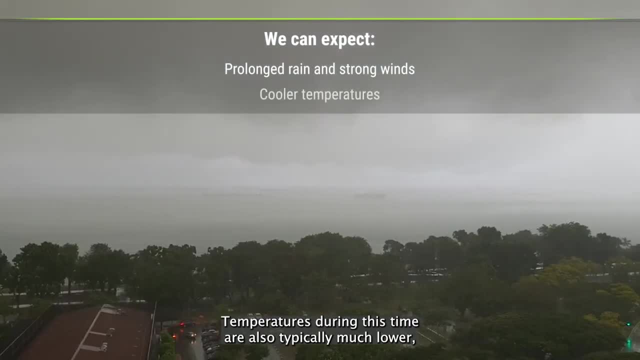 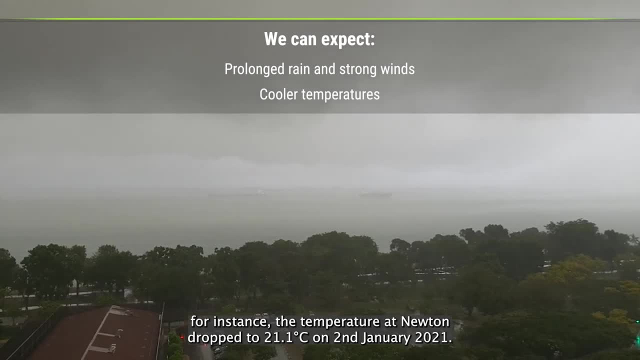 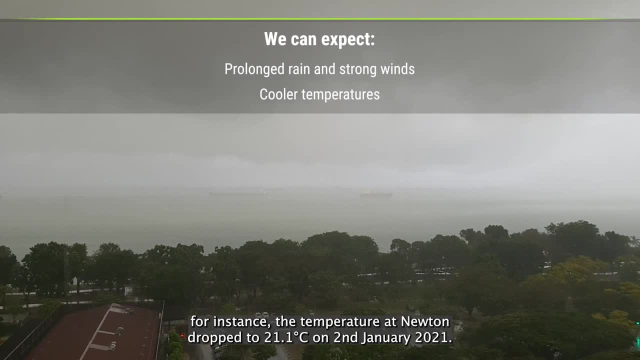 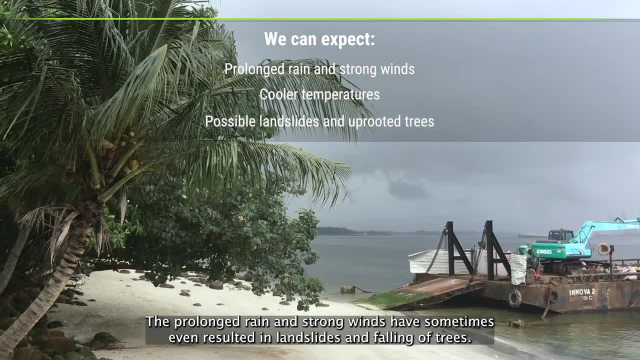 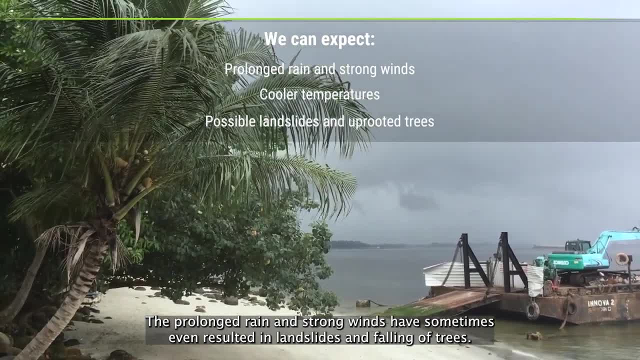 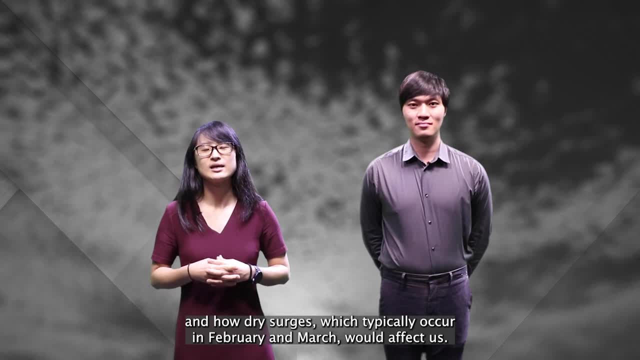 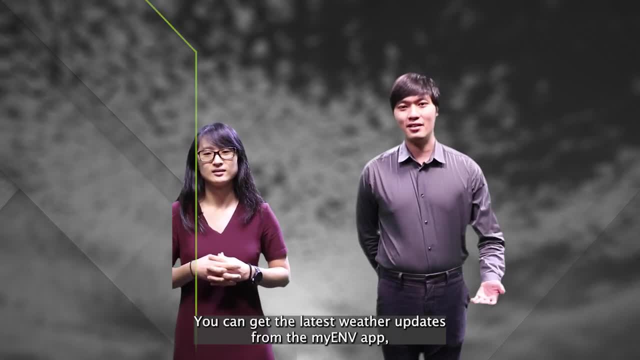 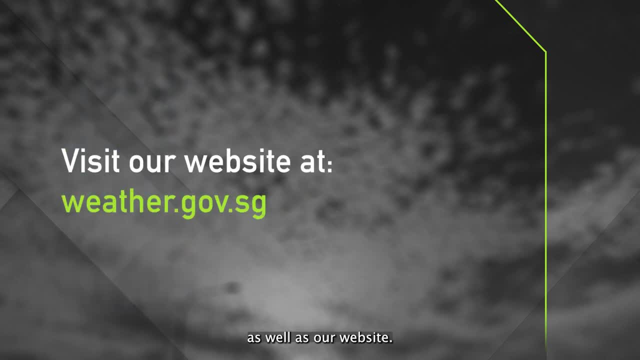 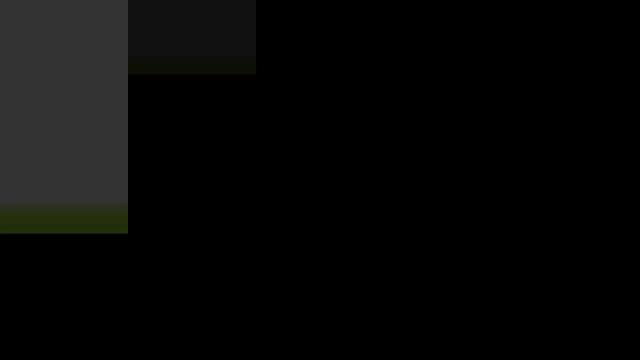